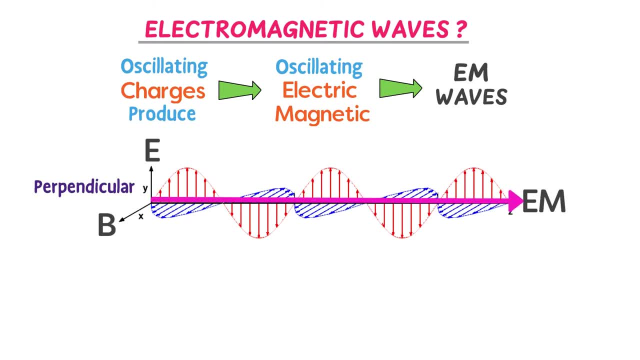 along Z direction is also perpendicular at 90 degrees to both electric and magnetic fields fields. Therefore we define electromagnetic waves as waves produced by the oscillations of electric field and magnetic field at 90 degree are called electromagnetic waves. Let me repeat it: Waves produced by the oscillations of electric field and magnetic field at 90 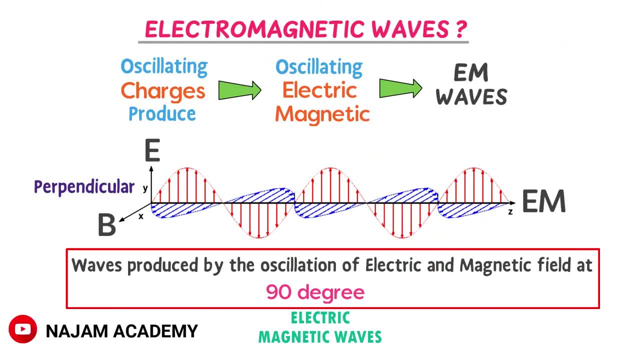 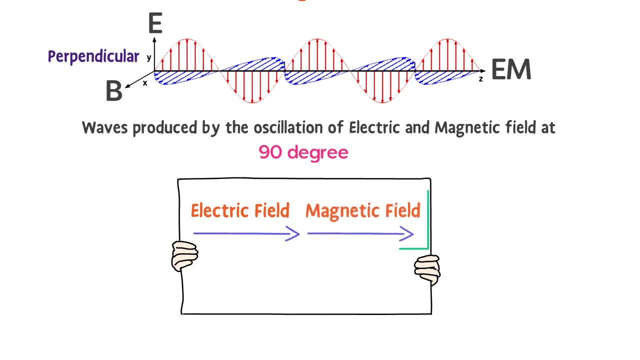 degree are called electromagnetic waves or EM waves. Here let me give you a bonus step: Can parallel oscillations of electric and magnetic fields make up an electromagnetic wave? Well, the answer is no. Parallel oscillations of electric and magnetic fields will not make. 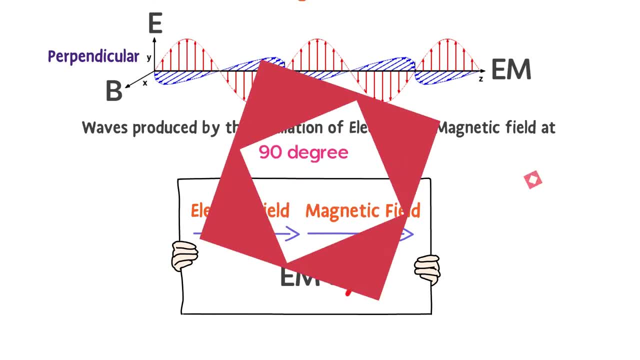 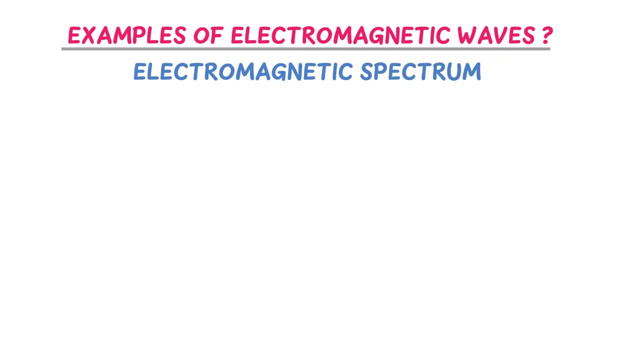 up electromagnetic waves. Now, what are the different examples of electromagnetic waves? is electromagnetic spectrum? well, the different examples are: electromagnetic spectrum is radio waves, microwaves, infrared visible light, uv or ultraviolet x-rays and gamma rays. they all are electromagnetic waves, are em waves. this group of electromagnetic waves are also commonly known as 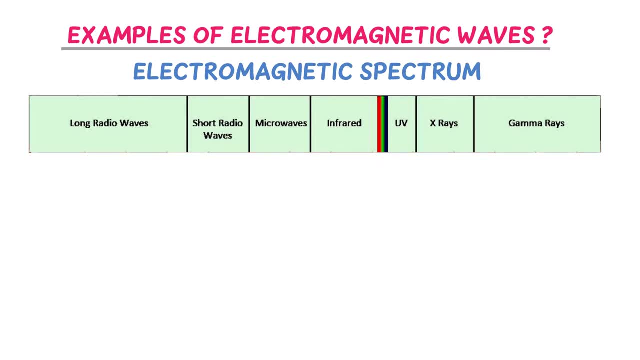 electromagnetic spectrum. now here, you should also learn that why electromagnetic waves are called transverse waves. well, noted down that these waves are transverse waves. it is because these waves travel in successive series of crust and trough. secondly, the oscillation of electric and magnetic fields are perpendicular to the wave motion, so electromagnetic waves are. 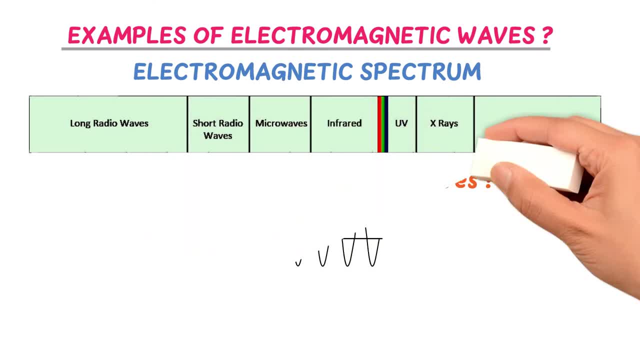 called transverse waves. remember that electromagnetic waves travel both in the medium and in the space, are in the vacuum. it means that they can transfer energy from one place to another place and the vacuum the sunlight we receive travels through the space. the speed of all electromagnetic waves is round about three and to ten. rest to the power, eight meter per second. 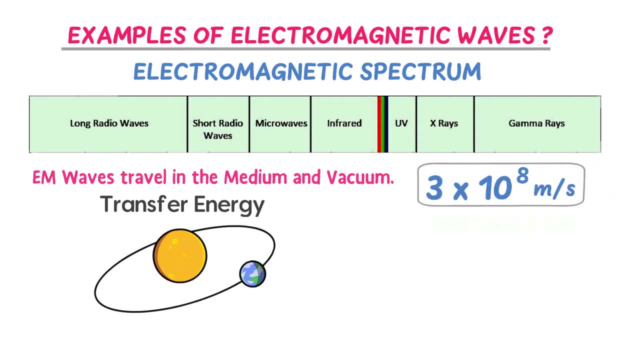 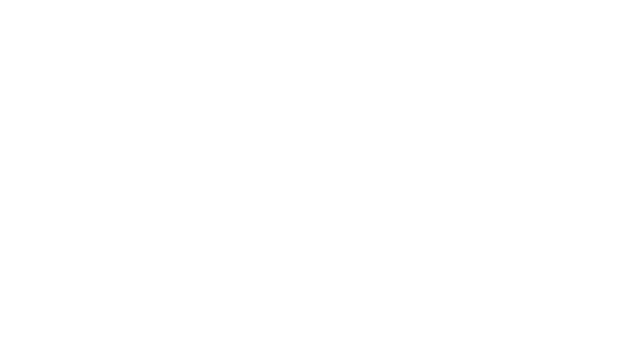 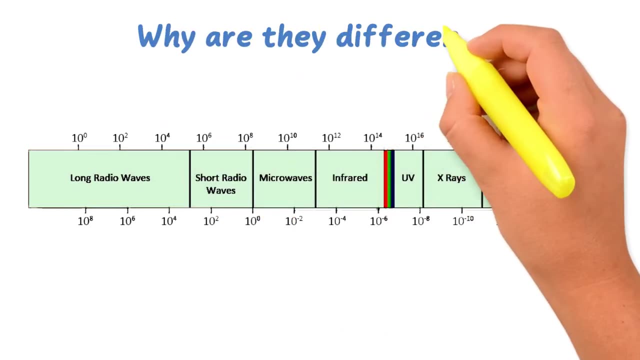 but this speed of electromagnetic waves vary in different media like solid, liquid and gas, due to diffraction of waves. here let me ask you: if these all are electromagnetic waves, then why are they different from each other? well, the answer is very simple: it is because of wavelength. 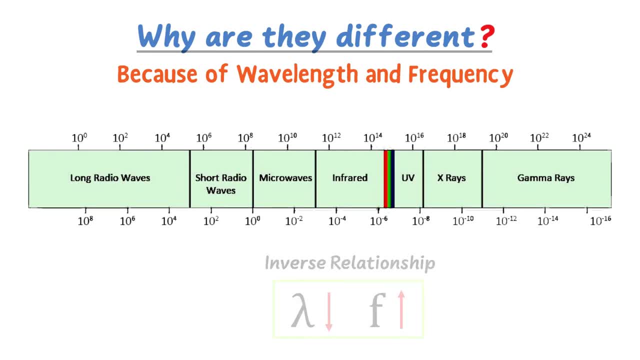 and frequency. we know that there is inverse relationship between them. if you increase the frequency, wavelength decreases, and vice versa. now listen carefully. radio waves are different from microwaves. it is because both the frequency and wavelength of radio waves are different from the microwaves. similarly, x-rays are different from gamma rays due to different 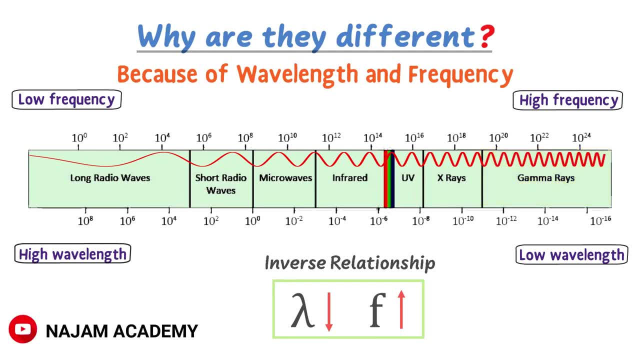 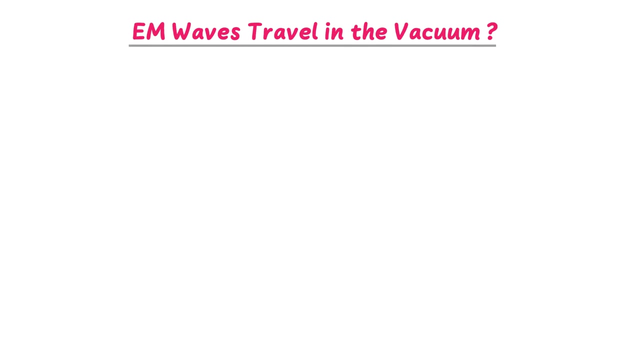 frequency and wavelength. for instance, when you go from radio waves towards gamma rays, frequency increases and wavelength decreases. therefore, we say that electromagnetic waves are different from each other due to having different frequencies and wavelengths. finally, let me teach you that how electromagnetic waves travel in the space are in the vacuum. well, we know that electromagnetic waves are nothing but the 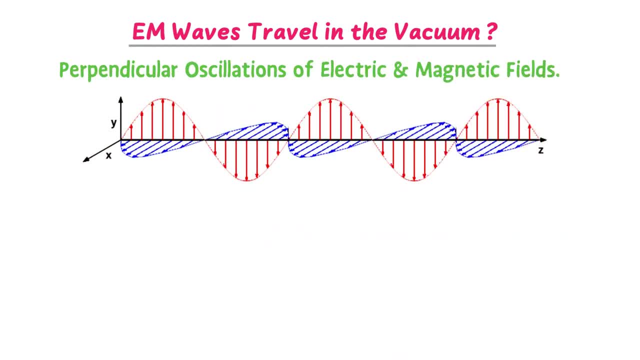 perpendicular oscillations of electric and magnetic fields means that electromagnetic waves generates because of this perpendicular oscillations of these two fields. now there are different theories that explain how electromagnetic waves transfer energy in the space, but the most easy is that when electromagnetic waves travel in the vacuum, are in the space, energy transfer from the electric 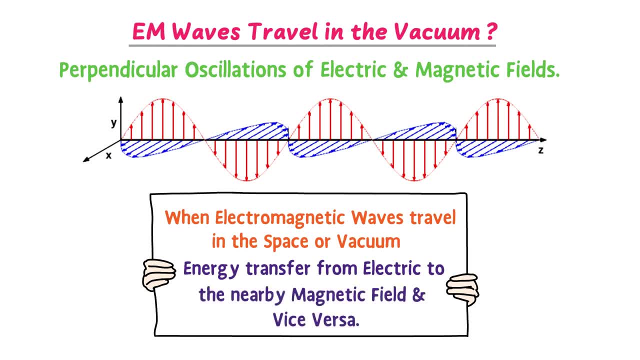 field to the nearby magnetic field, and then this energy transfer from the magnetic field to the nearby electric field. this cycle repeat itself in the space and acts as a electromagnetic pendulum and the space. thus energy is transferred from one place to other place. you so, by this way, electromagnetic waves travel in the space. this was all about. electromagnetic waves.